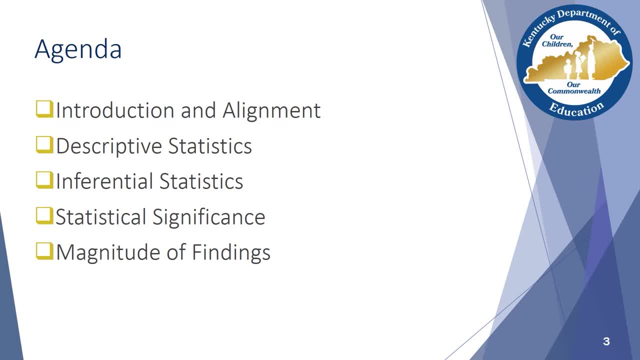 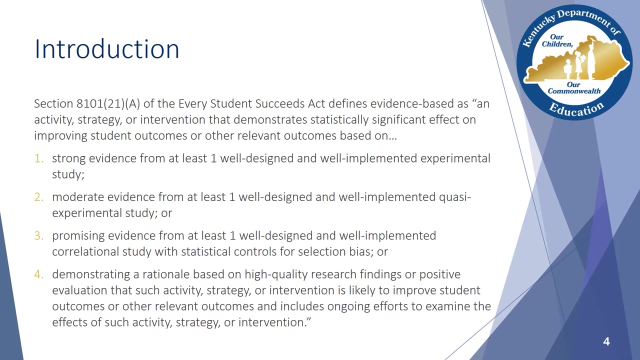 Then we will provide an overview of descriptive and informative information. Then we will provide an overview of statistical significance and interpreting the magnitude of a finding. In 2015,, the US Congress passed the Every Student Succeeds Act, or ESSA. This law reauthorized the Elementary and Secondary Education Act and created new mandates for school improvement efforts across the country. 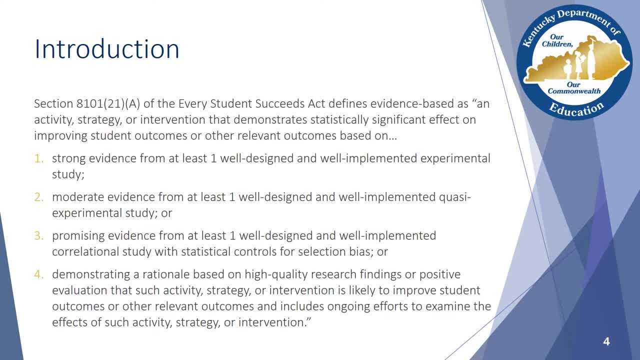 One of those new mandates is that processes, practices, products and strategies used for turnaround efforts be rooted in school improvement. ESSA defines four levels of evidence, each with the requirement that studies demonstrate statistically significant or substantively important improvement on the student outcome. 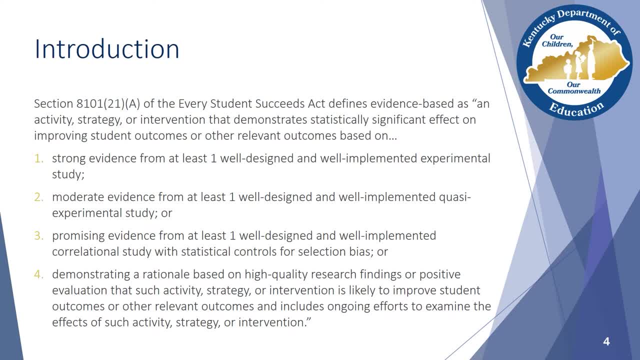 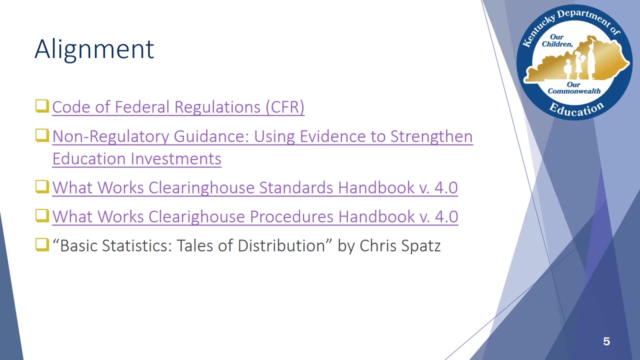 In this webinar, we will present information related to common statistical tests to support educators as they seek to interpret and apply research findings in schools and classrooms. Effort has been made to ensure that the definitions and key concepts presented in this webinar align to multiple educational regions. 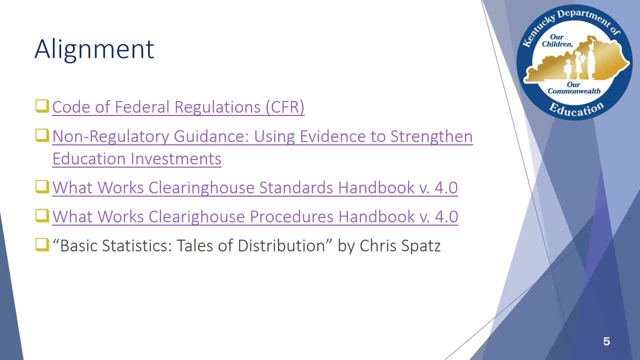 Thank you. We will continue to do this work to make the resources available to our students and our educators unique and relevant to education. Those references include the Code of Federal Regulations, the non-regulatory guidance Using Evidence to Strengthen Education Investments, the What Works Clearinghouse Version 4.0 Standards Handbook and the What Works Clearinghouse- Version 4.0- Procedures Handbook. 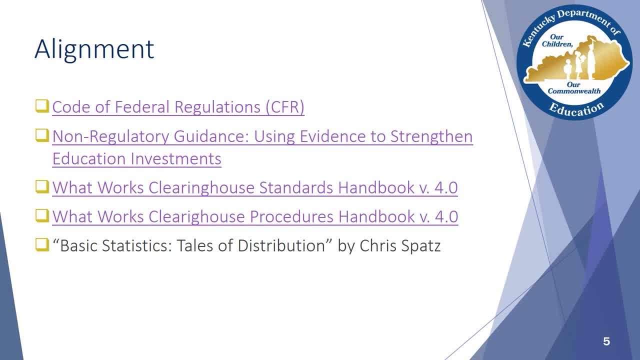 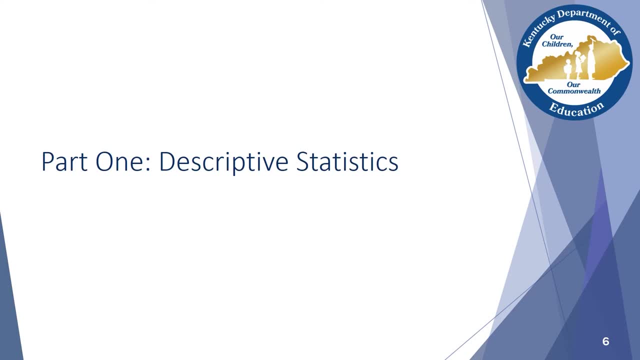 Obviously, these resources have been hyperlinked in the PowerPoint for your convenience. General definitions and interpretations for this webinar can be attributed to the book Basic Statistics- Talents of Distribution by Chris Spatz. We will begin our discussion today with descriptive statistics. Descriptive. 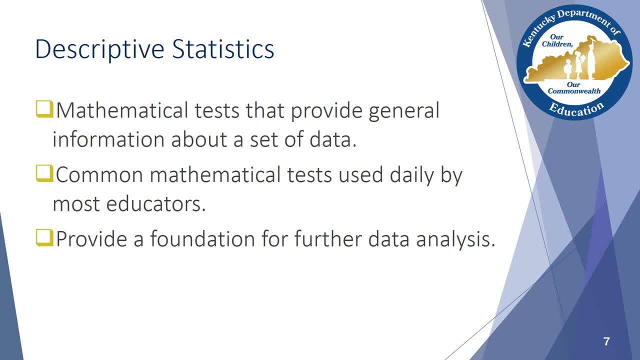 statistics are mathematical tests that tell us general information about a body of data. They are generally well understood by most educators and include very common tests such as average, median and standard deviation. Descriptive statistics usually provide a foundation that can be used for further analysis by 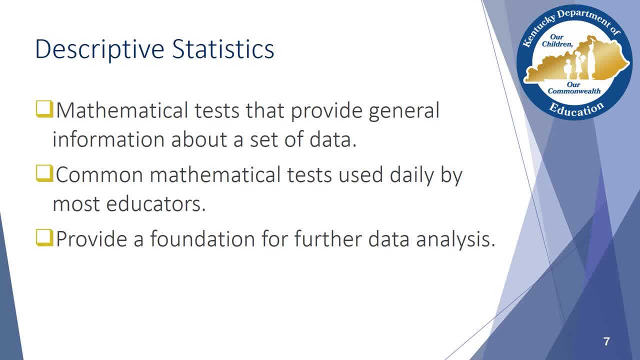 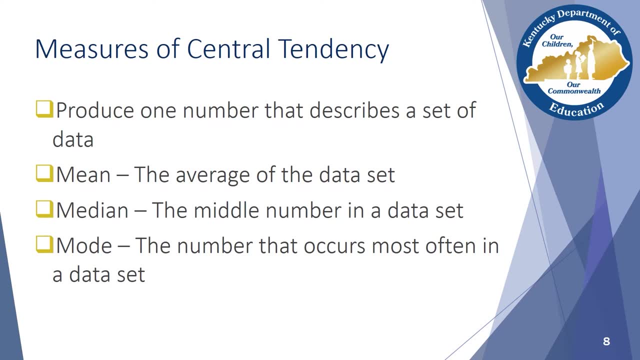 more complex statistical tests and therefore will be included in most research studies. The most common set of descriptive statistics are a classification called measures of central tendency. These measures produce a single number that describe a data set. There are three primary measures of central tendency: mean, median and mode. The mean represents the average of a set. 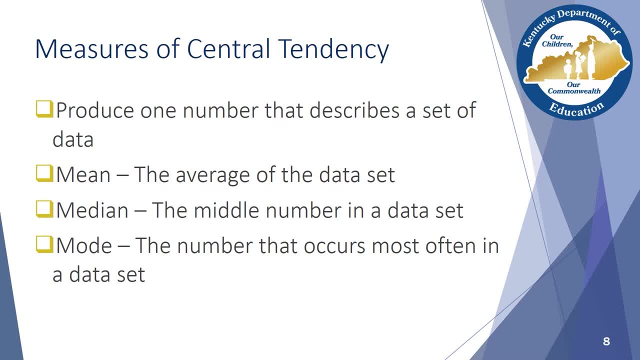 of scores, or the sum of the scores divided by the number of scores. The mean is a valuable measure that tells us generally how well a group of students performed on an assessment or how well a single student performed on a group of assessments. The mean is the formula used by most educators to 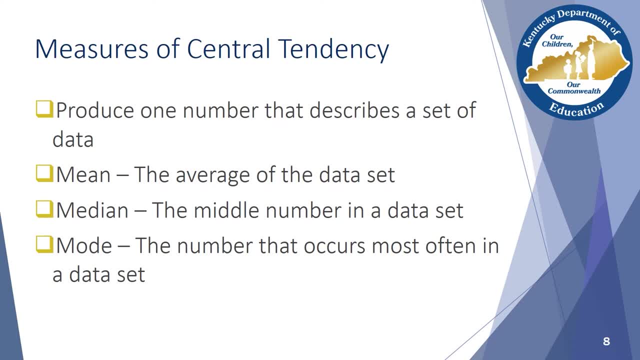 calculate grades at the end of the term. Later in this webinar we will discuss how the mean can be used to draw further conclusions about a body of data. The median represents the middle number in a distribution of scores. To find the median, the study author places the scores in ascending order from lowest to 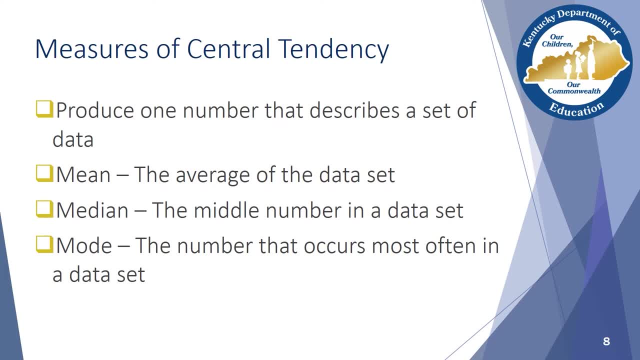 highest and then finds the middle. If there is no middle score, the average of the two center scores is calculated to determine the median. In other words, the median represents a hinge point where half of the students scored higher than the median and half of the students scored lower. Finally, the mode represents 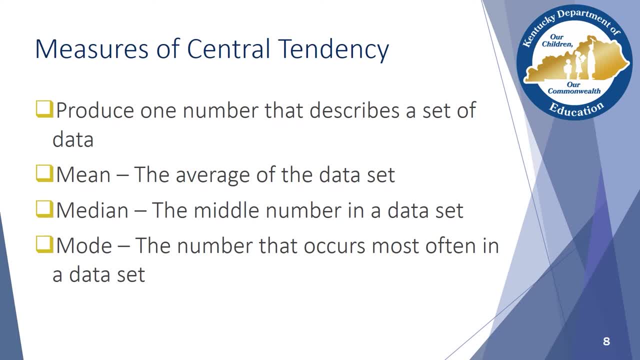 the score that occurs most often within a distribution of scores. This can be valuable in exploring clusters of students and discussing why they are or are not moving at the same rate of other students. A distribution of scores can have two modes, which is called bimodal, or three or 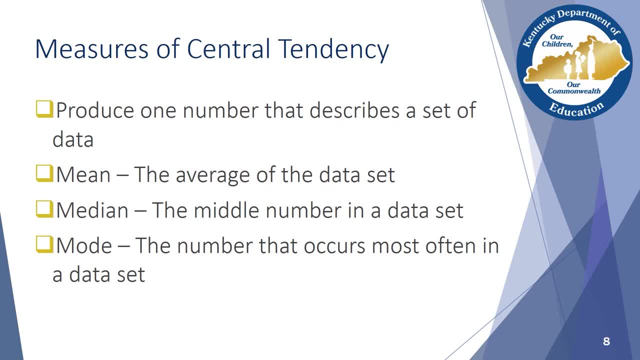 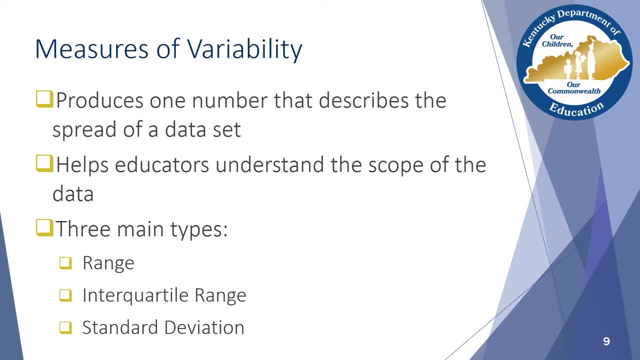 more modes, which is often called a multimodal distribution. Another common way to describe a data set is through measures of variability. Variability provides a single number that describes how spread out the scores in a data set are. This is valuable information for educators, who need to ensure that all 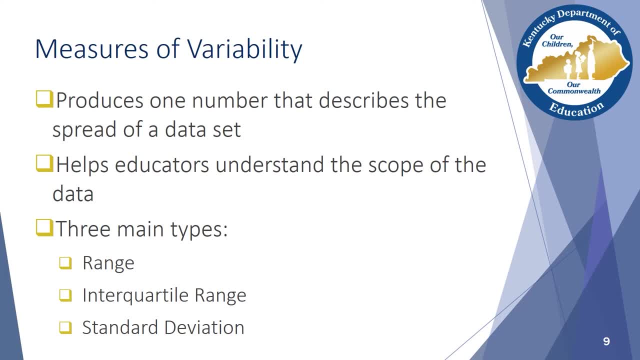 students are moving. Generally, when variability is low, students are moving as a group, whereas a data set with high variability may suggest that some students are moving at a high rate of variability. This is important to know faster or slower than others. There are three main measures of variability used. 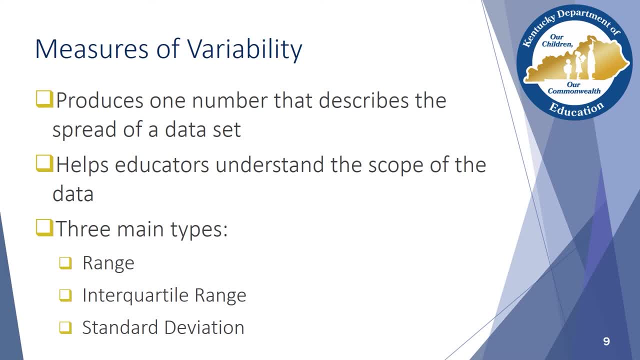 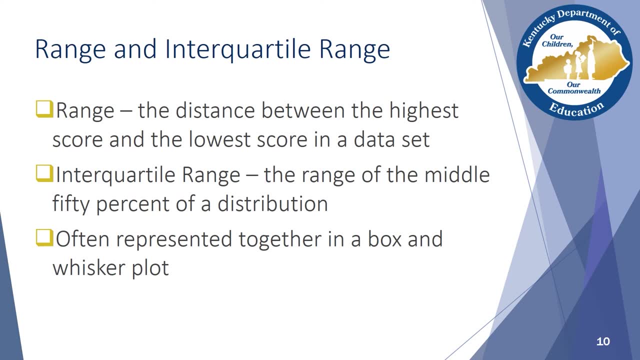 in educational research: the range, interquartile range and standard deviation. The range represents the distance between the highest score and the lowest score in a data set, While range represents a whole body of data. the interquartile range represents only the middle 50% of scores. Typically, 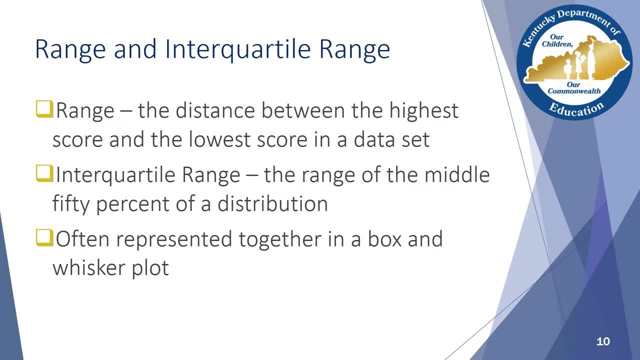 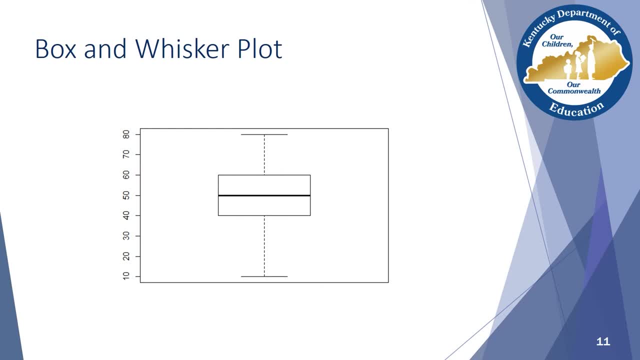 these two calculations are represented in a box and whisker plot. On this plot, the box represents the interquartile range, while the whiskers represent the full range of scores. A box and whisker plot will also typically indicate the median scores. for comparison, Let's pretend that the example on the screen 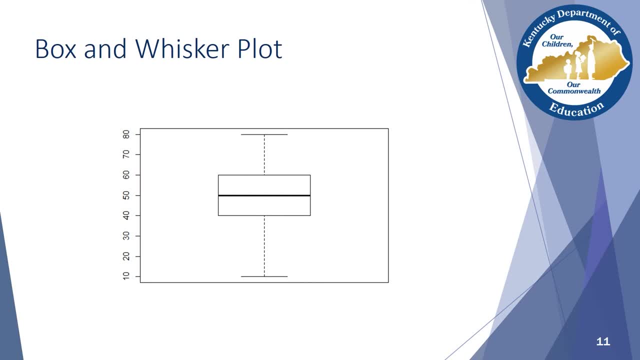 represents student test scores. You can see that there are roughly 70 points between the highest and lowest score plotted, while the median score is around 50. A plot such as this can help us see that 50% of our students, those represented by 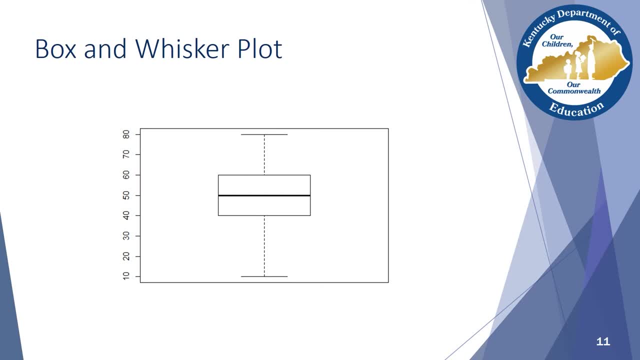 the interquartile range are clustered within 40 to 60% range, and we have at least one student who's dramatically outscoring the rest of the students in the group. Now, if this plot represents a pretest, we could place a post-test plot. 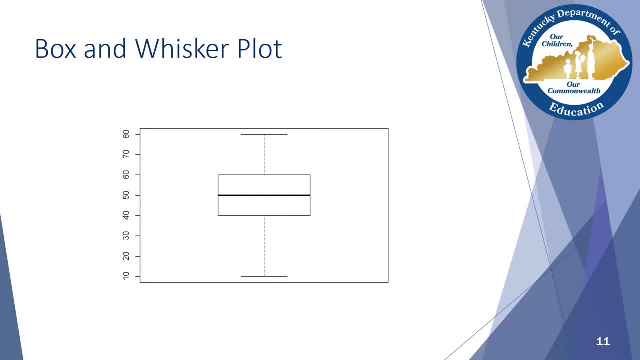 next to it to see how far our students have moved as a group after instruction or intervention. This plot gives us new information about how the students' performance on our fictional assessment. You can see that the class as a whole performed much higher on the post-test than the pretest The whiskers on the 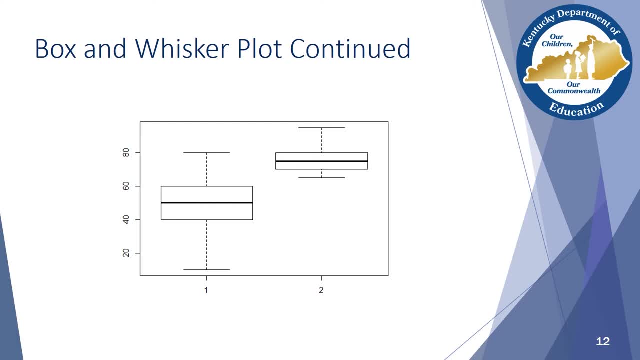 post-test plot representing the range are much shorter than on the pretest plot, telling us that the student scores are much closer together. We can also see that our median score has risen about 25% and the outer edges of the box representing our interquartile range are closer to the median. This suggests that 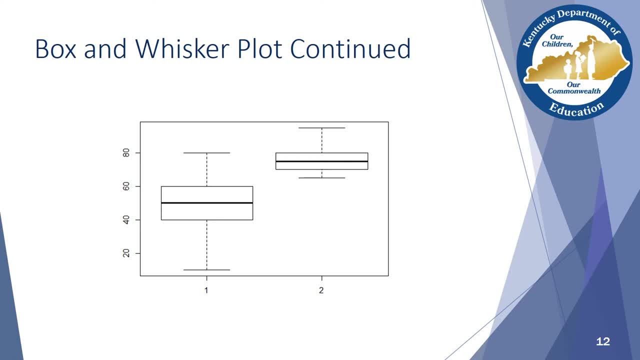 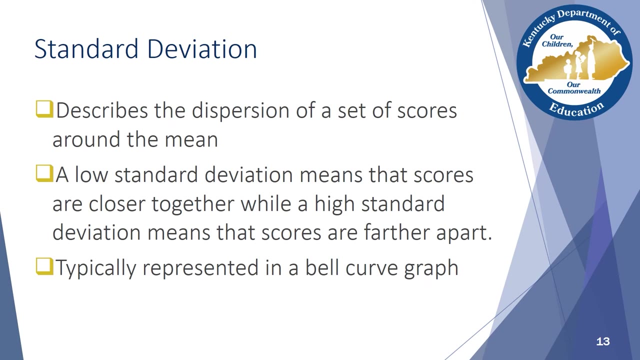 50% of our students are scoring closer to the median than before. This is a good example of this. Graphic representations such as this are very common in reporting educational research. Standard deviation is another common measure of variability, Like range. it helps us understand how spread out the data is. 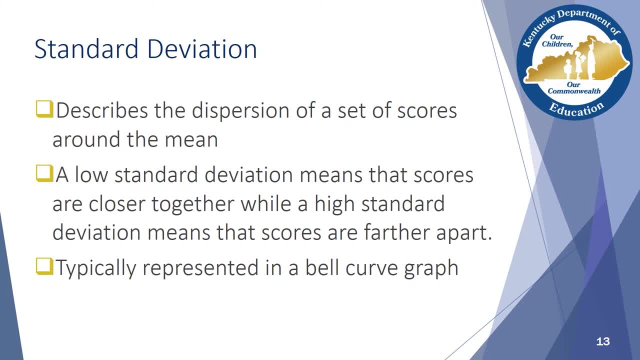 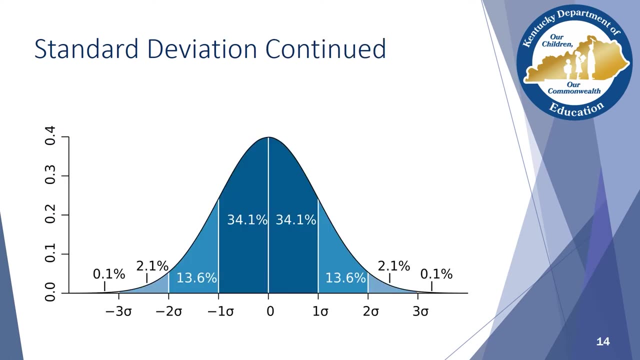 but it goes a step farther by exploring how the data is distributed around the mean. When a standard deviation measure is low, it means that the scores are clustered around the mean, while a higher standard deviation means that the scores are more spread out. Standard deviation is represented graphically with a bell curve like the. 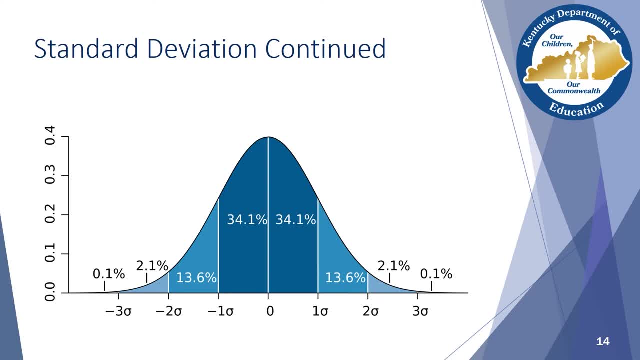 chart on the screen. The tall vertical line in the middle, labeled zero on this chart, represents the mean. You can see that in this example, 34.1% of scores fall within one standard deviation of the mean in either direction. This means that roughly 68% of scores are clustered together near the 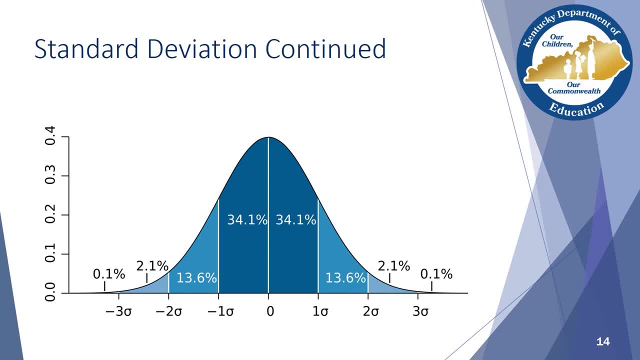 mean. As you move farther away from the mean, we see that 13.3% of scores are one standard deviation away from the mean, 2.1% of scores are located two standard deviations from the mean, and so on. Standard deviation is an. 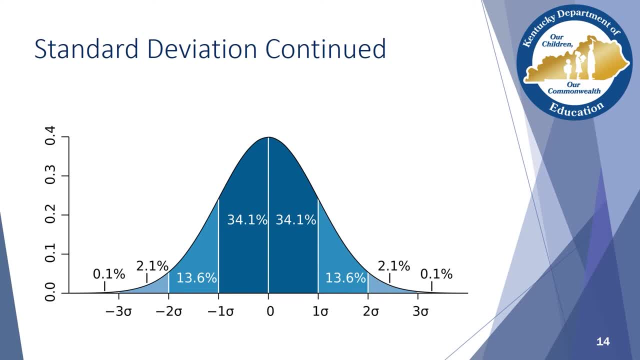 important measure for educators because it helps us not only see how spread out our student scores are, but also how far away from the mean different groups of students may lie. For example, a teacher may assign students who scored two standard deviations above the mean to enrichment activities, while students who 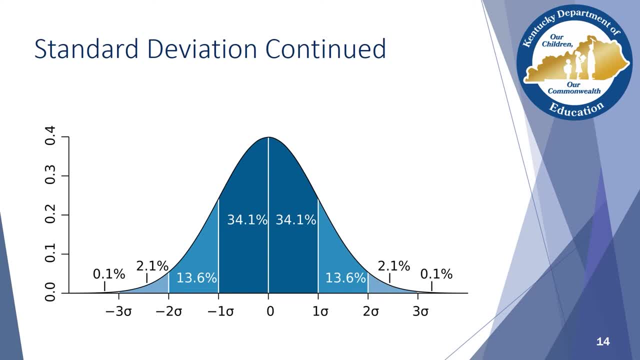 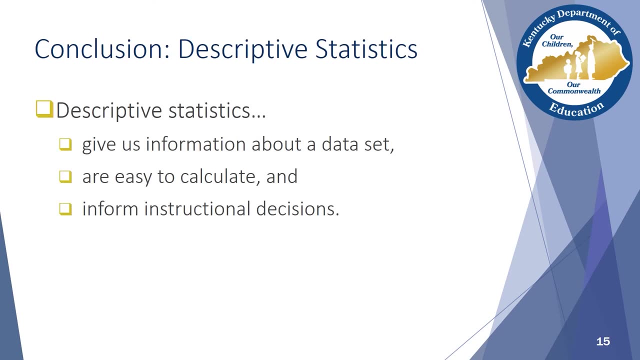 scored two standard deviations below the mean may be assigned two standard deviations to enrichment identified for intensive intervention. This type of grouping is one way that education research may assign students to groups. This is an assignment method called stratification. Altogether the descriptive statistics discussed in this 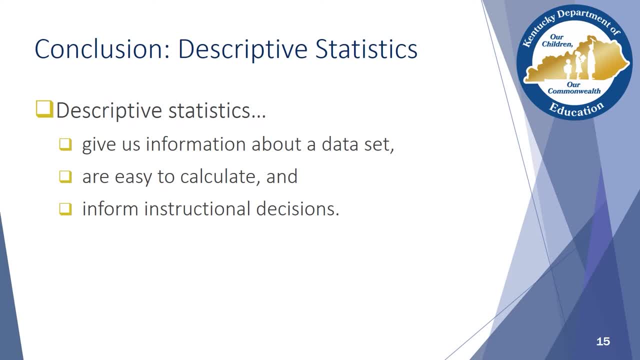 webinar help educators and education researchers to gain a general understanding of a body of data. These easily calculated statistical measures can be used to explore student performance and make instructional decisions. Next we will see how descriptive statistics can be used to further make inferences from the data. Let's stop here to check for. 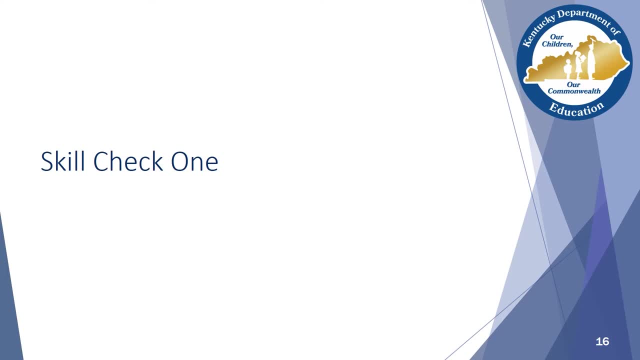 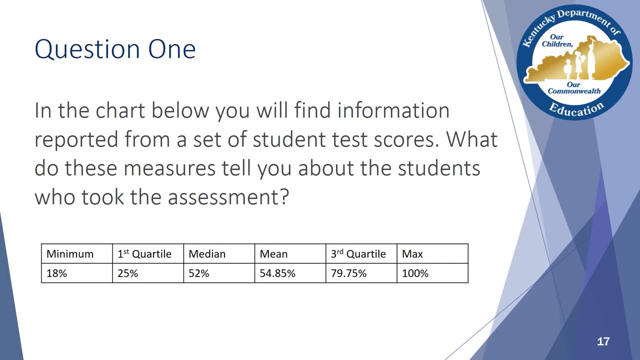 understanding. On the slides that follow, you will be asked to interpret the findings of three statistical tests. Question 1. In the chart below you will find information reported from a set of student test scores. What do these measures tell you about the students who took the assessment? 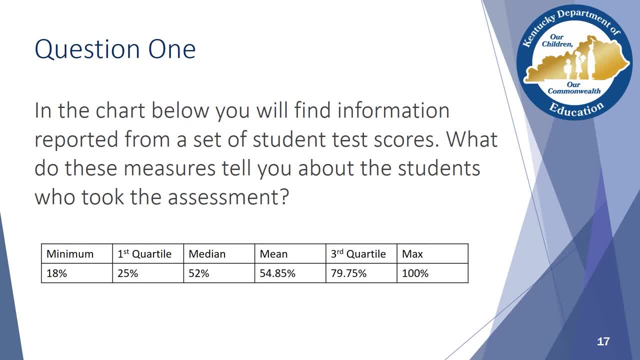 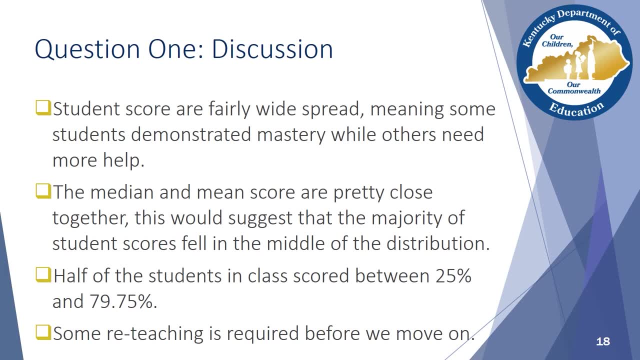 Postpone the assessment. If you have any questions, please feel free to ask them in the Q&A box below. Pause the webinar now and replay when you are ready to hear the discussion. Now that you have had a chance to look at the data, let's talk about what it. 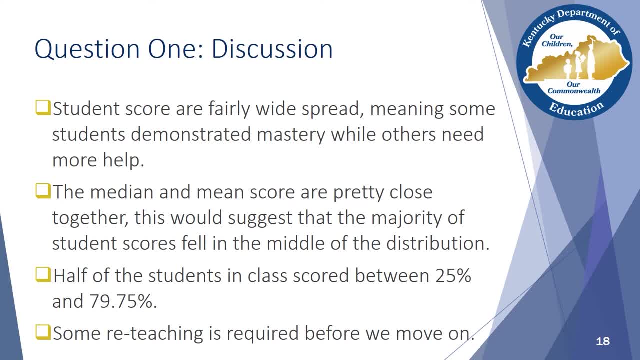 tells us? First, we can look at the spread of the scores. Here the scores are pretty widely spread from 18% to 100%. This tells us that some students demonstrated mastery, while others still need help. The median or middle score and 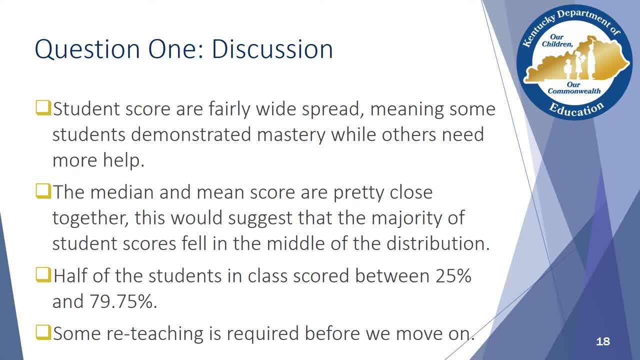 the mean or average are pretty close together. That tells us that the majority of our students fell near the middle of the distribution. We also know that half of our students scored between 25% and 79.75%, Assuming a mastery score is 80% or above. this tells us that the 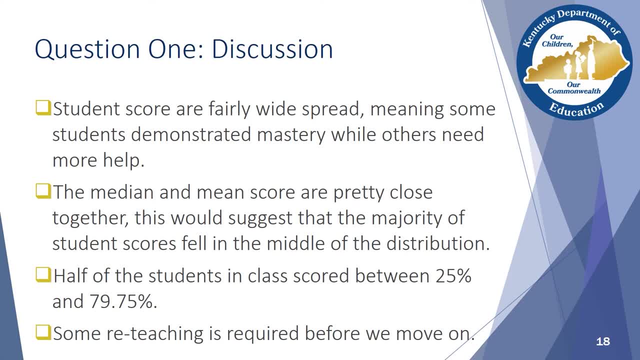 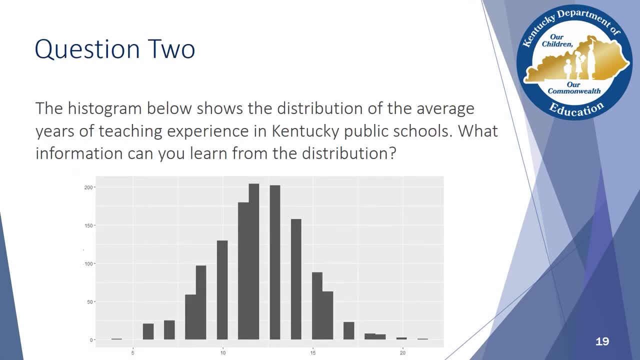 majority of our students missed the mark and some reteaching is required. Question 2.. The histogram below shows the distribution of the average years of teaching experience in Kentucky public schools. What information can you learn from the distribution? Pause the webinar now and replay when you are ready to hear the discussion. 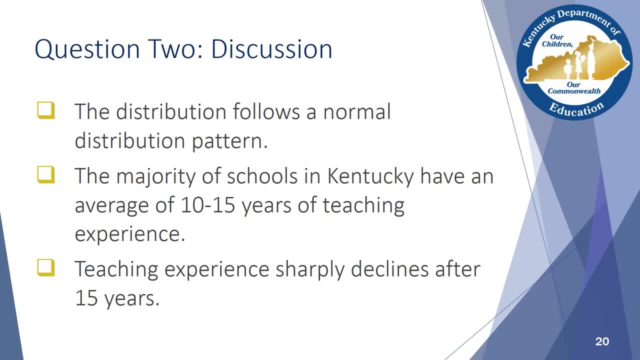 A histogram shows the distribution of a set of scores. Since this distribution looks similar to the bell curve we discussed earlier, we know that this dataset follows a normal distribution pattern. In other words, the data fell the way that we would expect it to. We also know: 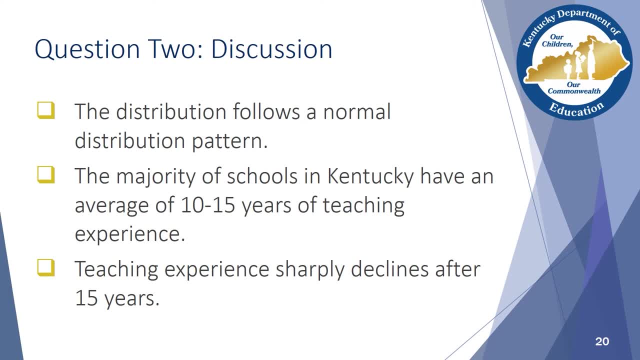 that the majority of schools in Kentucky have a teaching staff with an average experience of 10-15 years, because the highest bars fall within that range. You may have noticed that the average years of teaching experience in schools drop sharply after 15 years. A next step may be to look at which schools have very high average teaching. 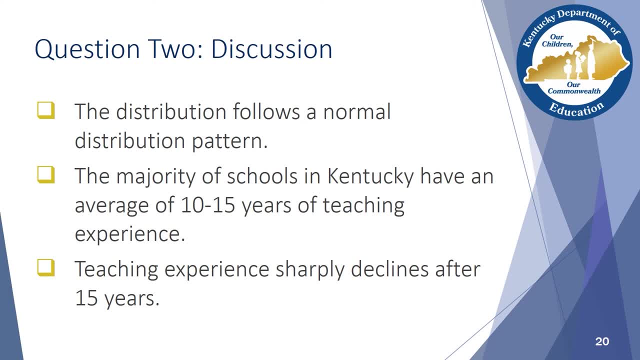 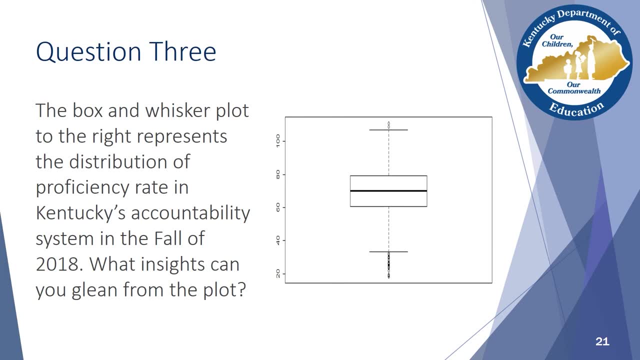 experience and see what other characteristics in those schools contribute to the longevity of their teachers. Question 3. The Box and Whisker plot is a very broad distribution of proficiency ratings in Kentucky's accountability system in the fall of 2018.. What insights can you glean from the box plot? 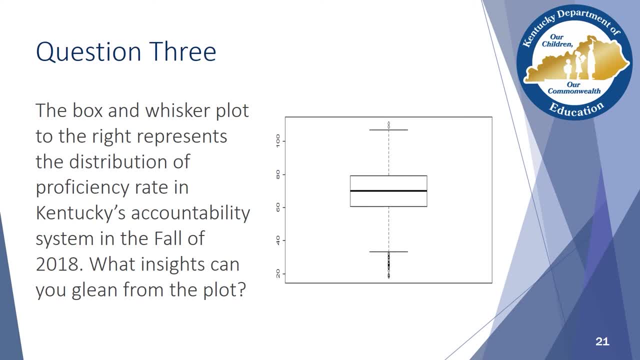 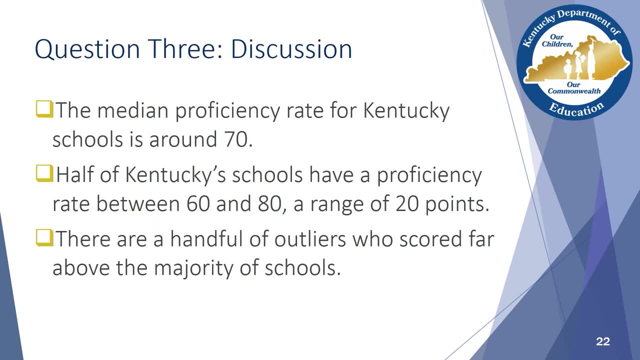 Pause the webinar now and replay when you are ready to hear the discussion. Remember that a box and whisker plot gives you descriptive information about a dataset. The bold line in the middle represents the median. Here we can see that the median proficiency rate for all schools in Kentucky is around 70%. 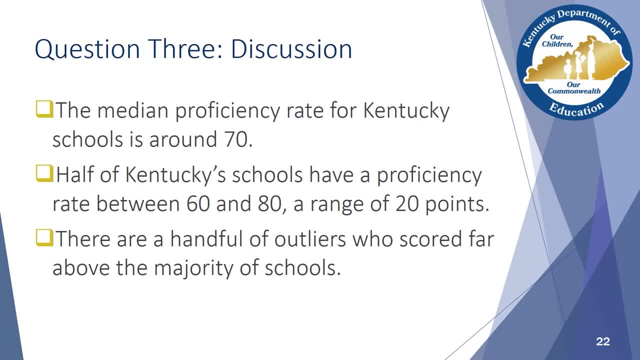 The box represents the middle half of scores. In this case we can see that half of Kentucky's schools fall within 60 and 80%, a range of 20 points. Finally, dots represent outliers. We can see that a handful of schools scored far above. 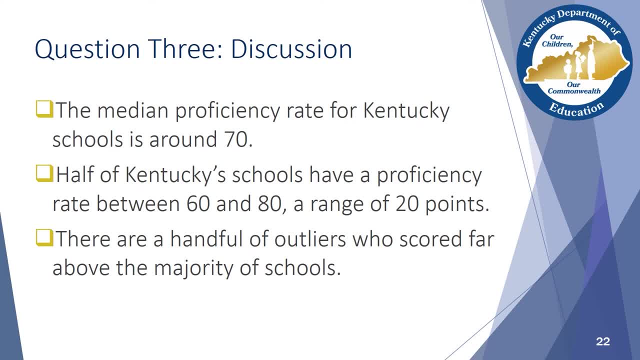 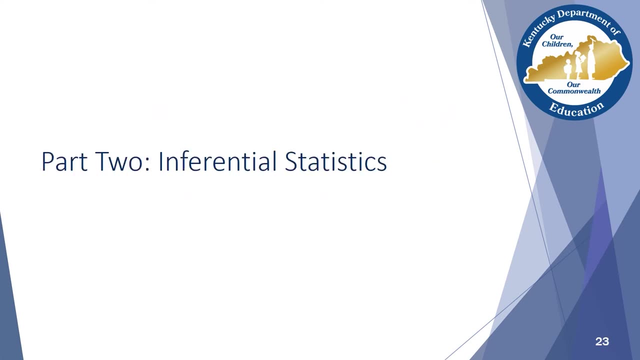 the majority of schools. If we were looking to improve our schools' scores, it may be beneficial to identify who those outlier schools are and examine the characteristics of those schools. Great work. We have explored the world of descriptive statistics and how they can be useful in analyzing a set of data. If descriptive 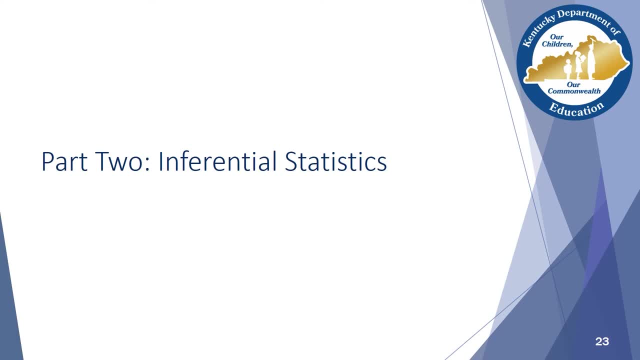 statistics gives us descriptive information of a dataset, then inferential statistics are those that allow us to make an inference or draw a conclusion from a set of data. In Part 2, we will explore a set of inferential statistics that are commonly found in education. 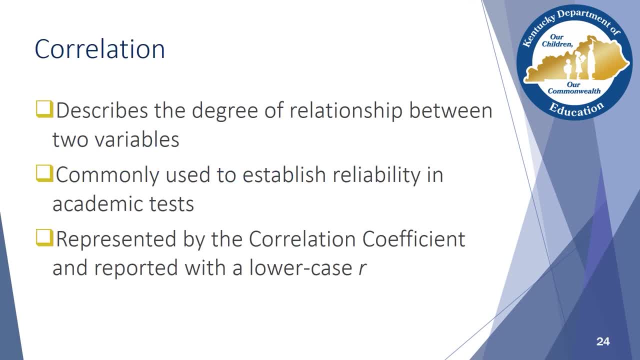 research. Correlation is arguably the most common inferential statistic used in educational research. That is because it can be used on its own to make an inference about a set of data, or combined with other tests to draw a more concrete conclusion. Correlation describes the degree of relationship. 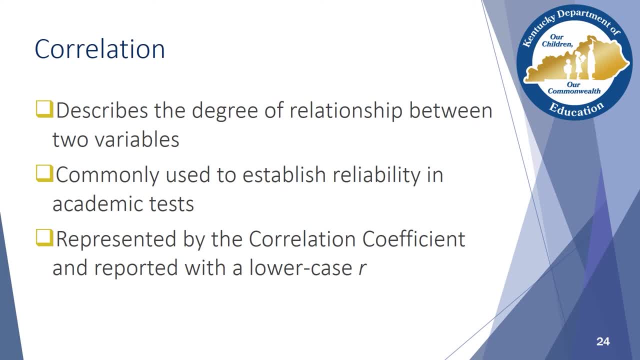 between two variables. It is used to answer questions like: is there a relationship between academic achievement and math and student gender, Or does household income impact student attendance rates? In addition to these simple comparison questions, we will also explore the relationship between the two variables. In Part 2, we will explore a set of inferential statistics that allow us to make an inference about a set of data. Or does household income impact student attendance rates? In Part 2, we will explore a set of inferential statistics that allow us to make an inference. 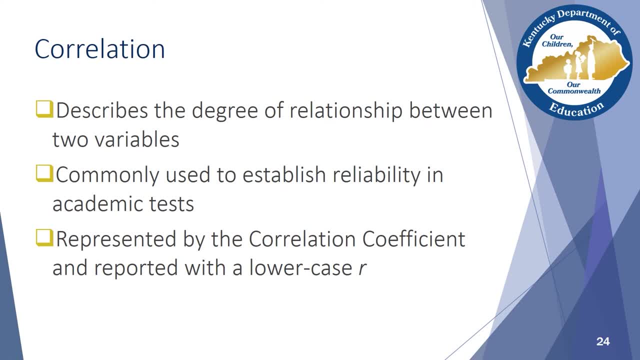 between two variables. Correlation is also used to determine the reliability or consistency of academic tests. In this model, a sample test is given to a group of students and then given to them again, without instruction in between. If the test is reliable, then the two sets of 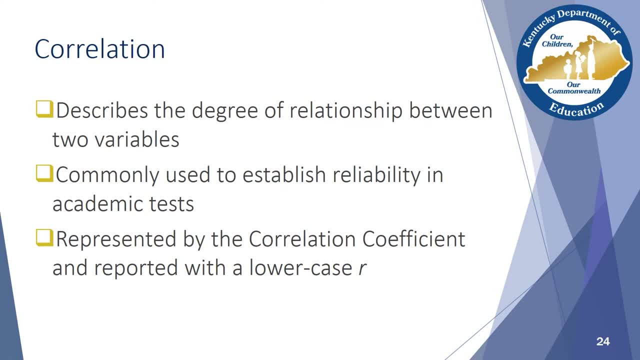 scores will have a high level agreement or a high correlation. If the test is not reliable, the two sets of scores will have a low correlation. This calculation is often seen in studies that use teacher-created assessments rather than established standardized tests- standardized assessments- in their collection protocol. When calculated, the 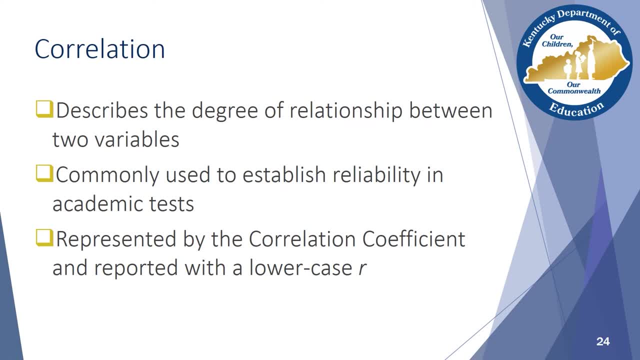 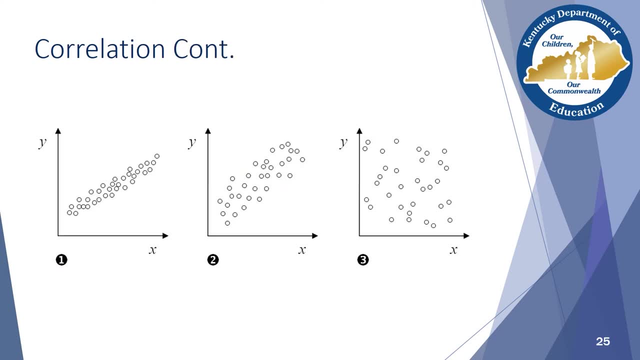 correlation is reported as a Pearson product moment correlation coefficient and is represented by a lowercase r. Correlation is graphically represented by a scatterplot. You can see three scatterplots on the screen. Scatterplot 1 represents a strong linear correlation. You can see that all the scores are clustered together and slope positively. 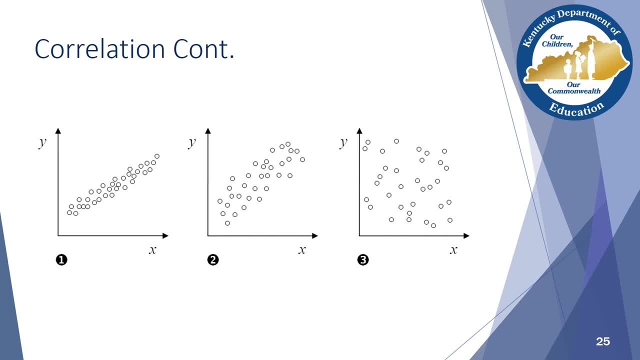 to the right. Plot 2 represents a weak correlation. In this plot, the scores slope positively to the right, but they are more spread out than in the first plot. Finally, scatterplot 3 represents a data set with no correlation. The data is not. 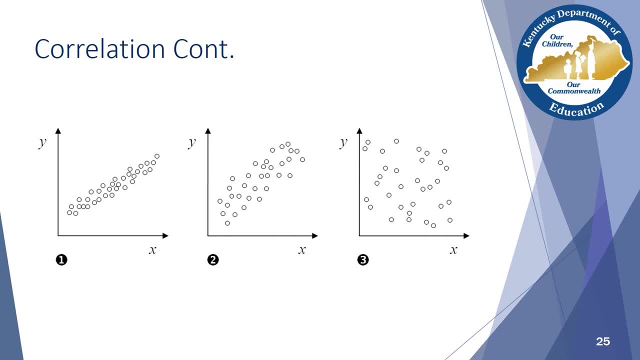 clustered, nor does it have a slope. While correlation can help us gain information about the relationship between two items, it cannot tell us if one variable directly influences another. For example, if we want to know the correlation between two items, we can use this example. If we find that low household income has a positive 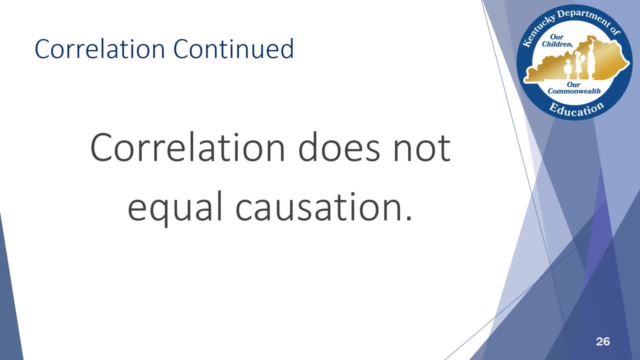 correlation with low student attendance, then we may want to direct some of our resources toward influencing the attendance of students from lower income households, But we cannot assume that having a low household income causes low student attendance. It is important that we interpret the results of correlational. 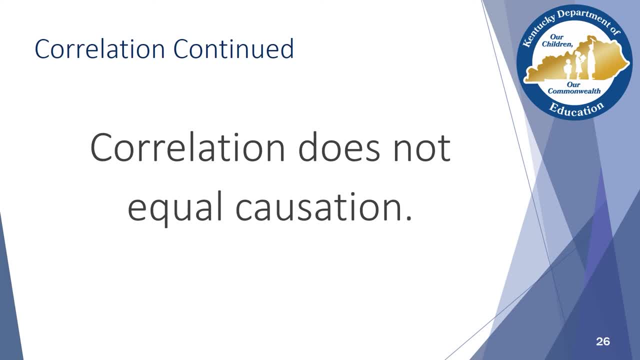 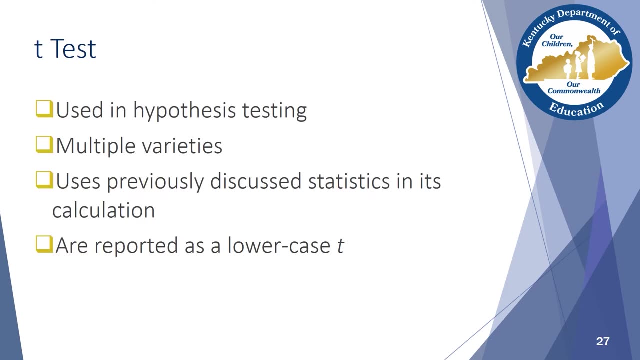 tests correctly when using them for education decision making. This test alone does not give us the whole picture, and the best practice would be to seek out specific data points to supplement this finding before committing time and resources towards a potential solution. When a researcher is trying to determine a causal relationship between two 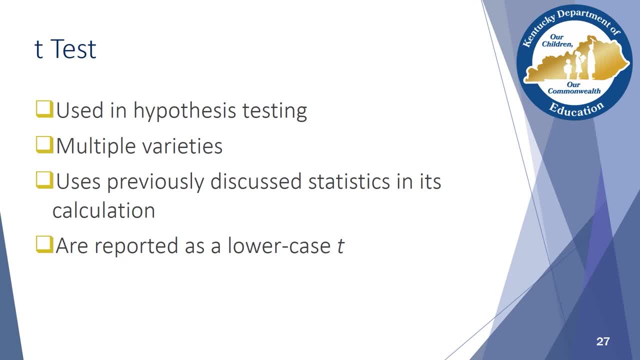 variables. the t-test is commonly deployed. The t-test is used in hypothesis testing or tests that seek to prove that one variable does or does not impact another variable. For example, a researcher may use the t-test to answer the question: does this intervention improve student scores on this assessment? The 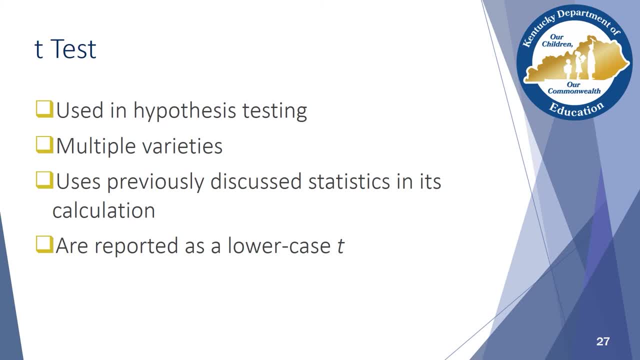 uses the data to examine a hypothesis and either reject or not reject the hypothesis. This is called the null hypothesis. Essentially, the null hypothesis is a hypothetical statement that the data may or may not support. It is common for researchers to write something like: this result rejects the. 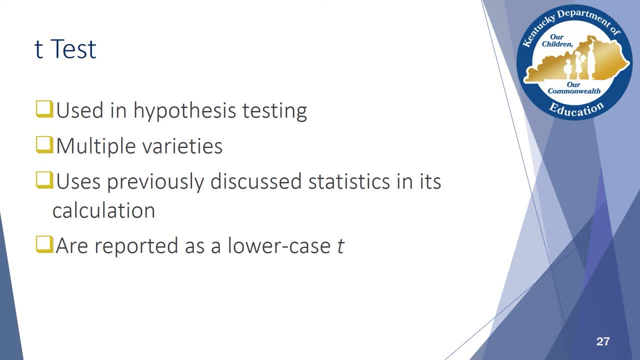 null hypothesis. to help put the results of a statistical test in context, The T test uses a variety of calculations already discussed in this webinar. The T test is, at its core, a comparison of mean scores, and some formulas will also include R or the correlation coefficient. The results of a T test are reported. 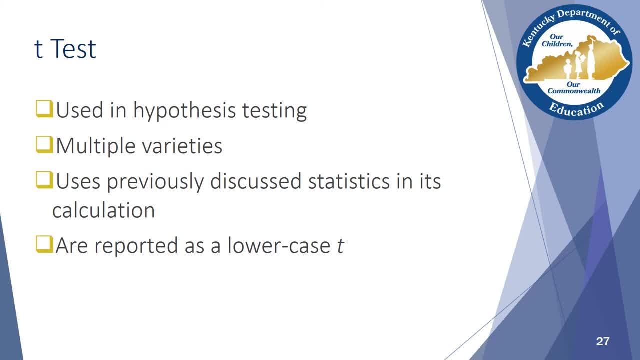 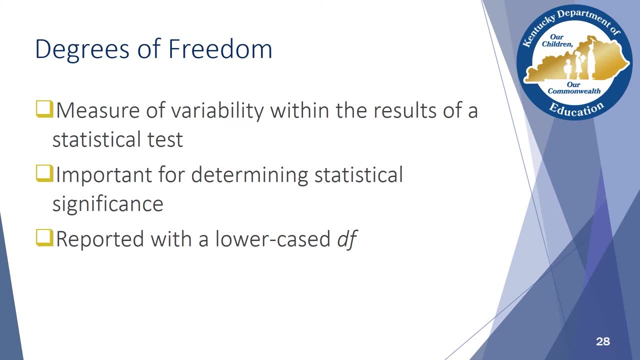 using a lowercase T. This is also a good time to introduce the concept of degrees of freedom. Similar to standard deviation, the degrees of freedom measurement tell us how much variability there may be within a result of a statistical test. This measurement typically reports as a lowercase D. F should be included in all T test results, as well as the. 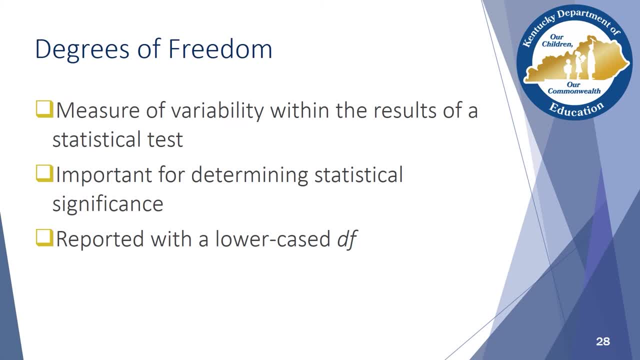 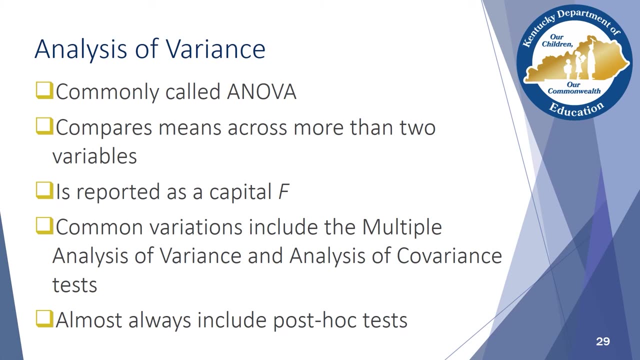 results of other common inferential statistical tests. This number is important for determining statistical significance, which we will discuss at the end of the webinar. The T test is a useful tool for researchers who want to compare two variables, but when more than two variables are necessary, they turn to. 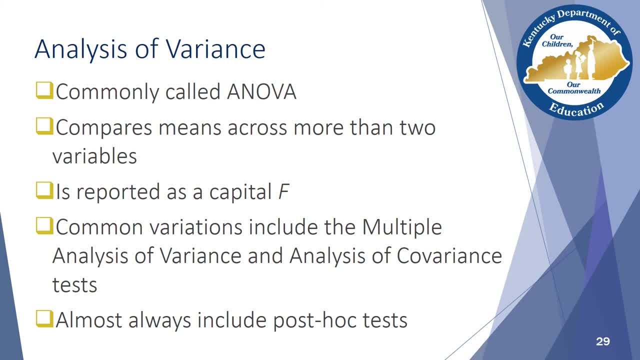 the analysis of variance test, commonly called a NOVA. Like the T test, a NOVA test is calculated using the means of a data set In education. an NOVA test may be used to answer questions like: do students from urban, suburban and rural districts 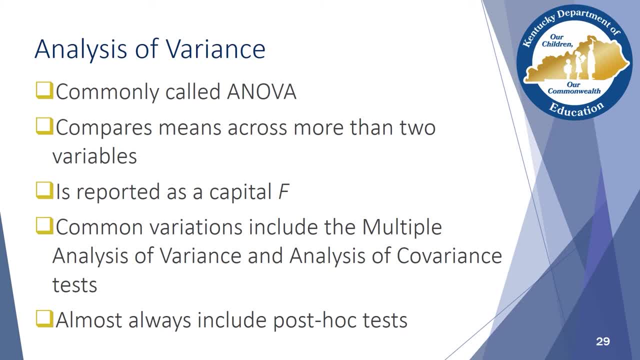 differ in their attitudes towards the importance of school. The NOVA test is reported as the F distribution, written as a capitalized F. You may see other variations of this test, such as multiple analysis of variance and the analysis of covariance. We will not do. 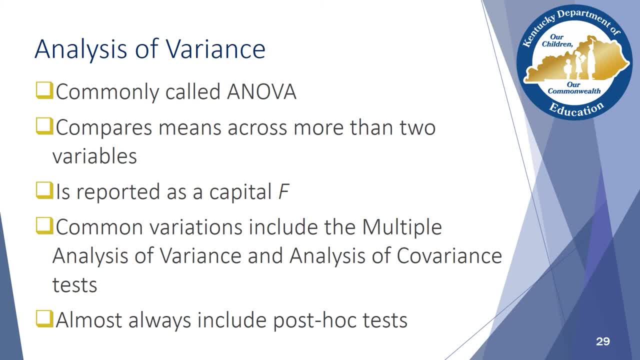 a full review of the analysis of variance. until we are done with this review, We will not explore the differences between these tests in this webinar. For our purposes, it is sufficient enough to know that these tests help researchers create more accurate findings. under certain conditions, The ANOVA test can tell you. 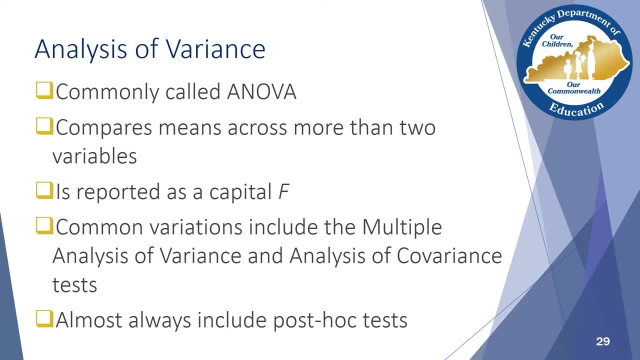 whether or not a relationship exists between variables, but it cannot tell you where those relationships lie. For that, researchers must deploy one of a variety of post hoc or after-the-fact tests to identify the specific relationship between variables. The final inferential test we will discuss in. 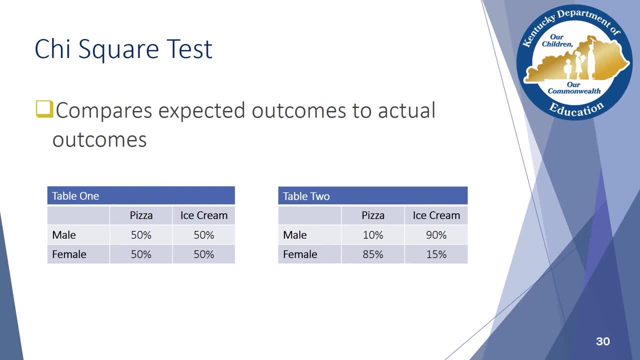 this webinar is the chi-square. The chi-square is used when we want to compare a data set with our expectations of a data set. Consider this hypothetical example: We ask a group of high school freshmen whether they wanted pizza or ice cream as a reward for on-time homework assignments. The result of that: 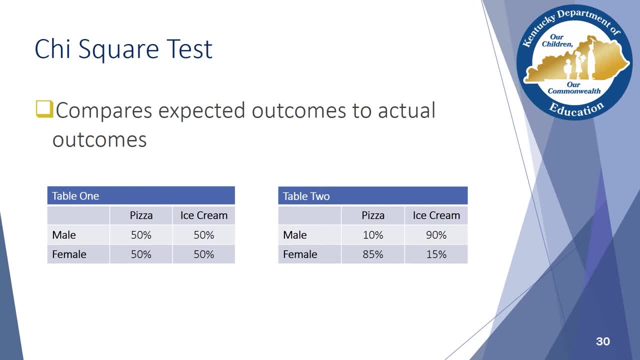 survey is on the screen, We might expect that the result will be split evenly between male and female. The results will be split evenly between male and female female students, as in Table 1.. If we found, however, that female students seemed to want: 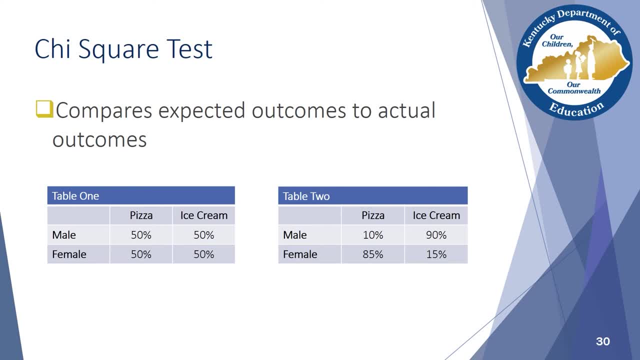 pizza and male students seemed to want ice cream. as you can see in Table 2, the chi-square test can help us determine if there is any statistical significance between gender and reward preference. In other words, the chi-square test tells us how confident we can be in making the statement. 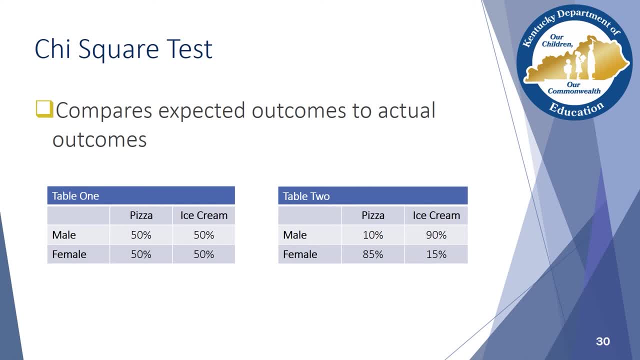 that there is a difference between our expected result and our observed result. While most education leaders would not conduct a chi-square test to determine reward patterns for on-time assignments, the chi-square method can be used by education researchers to answer much more serious questions that can impact policy decisions Any time the data can be broken down. 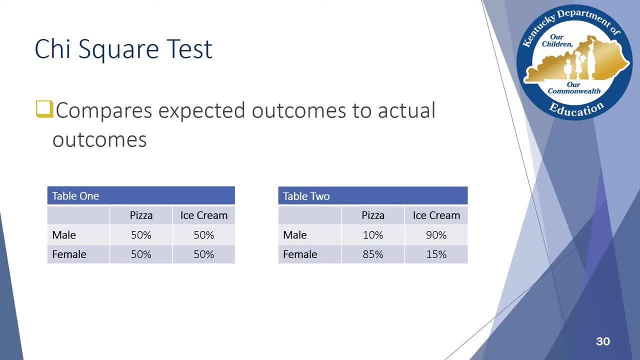 into a chart like the one on the screen. a chi-square can be used to draw a conclusion. For example, we may want to compare the opinions of parents who send their kids to public school versus those who send their kids to private school on a given variable, or compare the proficiency. 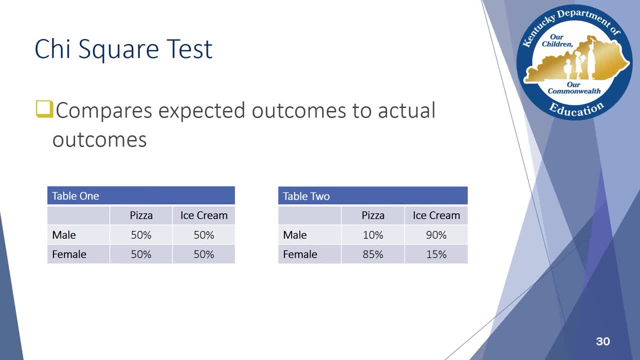 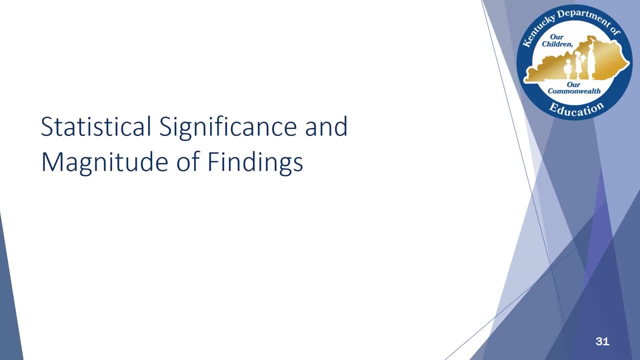 rate of students in schools with a population over 500. with schools in a smaller population. Inferential statistics help researchers draw conclusions about a set of data. They typically build off of the descriptive statistics discussed in the previous section of this webinar and provide greater insight into a population. So far, we have simply discussed 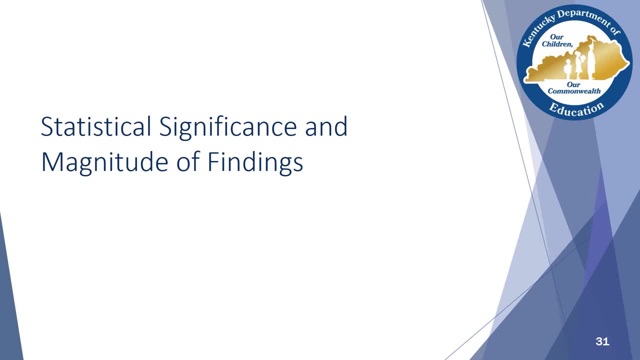 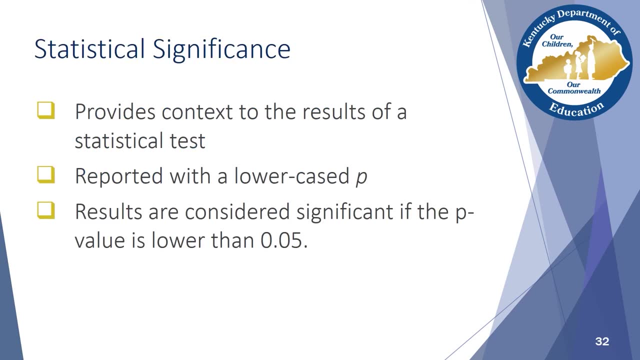 inputs and outputs. but now let's talk about how we know what those numbers mean. The result of a statistical test is simply a number until we give it some context. That is where measures of statistical significance come in. The significance of a statistical test is reported by the p-value, written as a lowercase p. 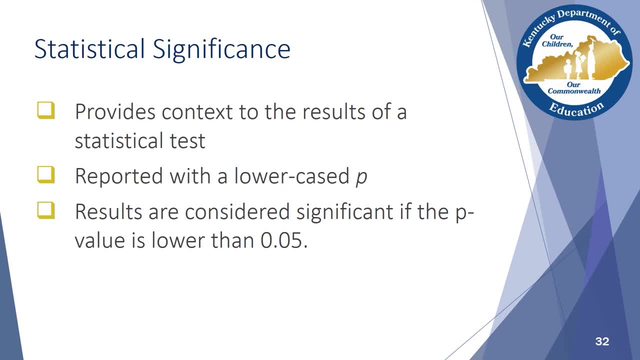 The p-value comes into play for all hypothesis tests and they tell us the probability of the statistical test value when the null hypothesis is true. For example, if you make a null hypothesis that says this intervention will improve outcomes for this student population, then the p-value tells. 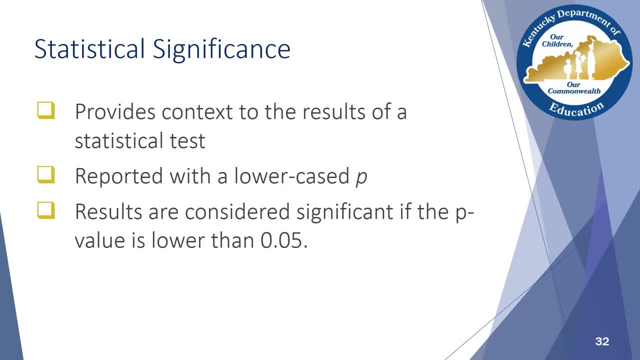 you the probability of the data observed If you make a null hypothesis. that says it is generally accepted that a statistical test is significant when it is less than 0.05, written as p less than 0.05.. If we apply this number to the null hypothesis stated a moment ago, 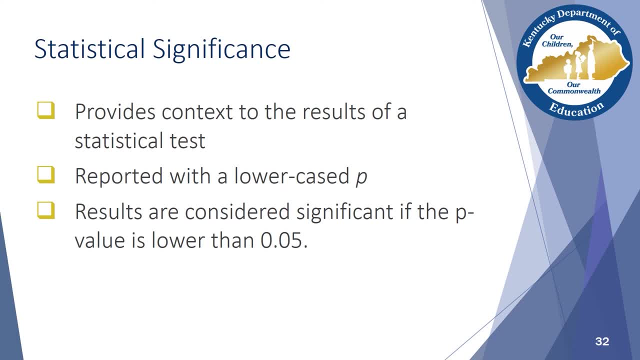 this would mean that the sample results you got would occur fewer than 5 times in 100 attempts. The p-value is considered highly significant if it is less than 0.01 or 0.001.. To determine the p-value, researchers compare the scores of their statistical tests. 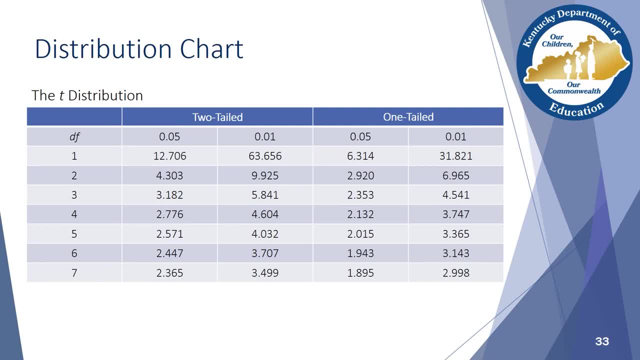 and the degrees of freedom to the distribution chart. like the one on the screen, This chart represents the first seven rows of a t-distribution table. These standardized tables are widely available and regularly referenced to by even the most senior statisticians. In order for a t-score to be significant, it must be equal to or greater. 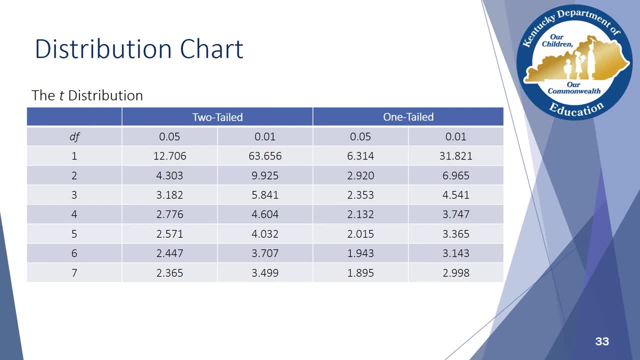 than the value shown in the column that aligns to the degree of freedom. For example, a t-score of t equals 5.64 with a degree of freedom measurement of 4 would be considered statistically significant with a p-value of 0.01.. 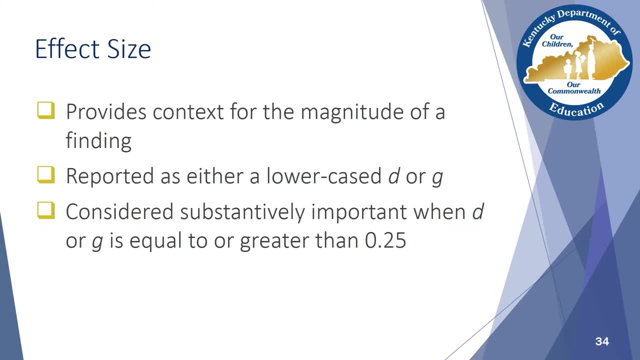 If the p-value tells you whether or not a statistical finding is significant, the effect size provides context as to the magnitude of a finding. The effect size compares the distance between the means of two datasets. In the pre-test- post-test model, the effect size would be calculated by subtracting the mean. 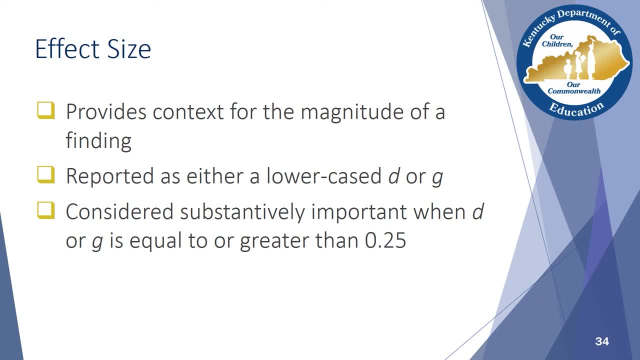 of the pre-test from the mean of the post-test and dividing by the standard deviation. This is how you tell how far apart two sets of scores are. Effect size can be calculated using either the formula for Cohen's d or Hedge's g, and is reported by a lowercase d or g respectively. 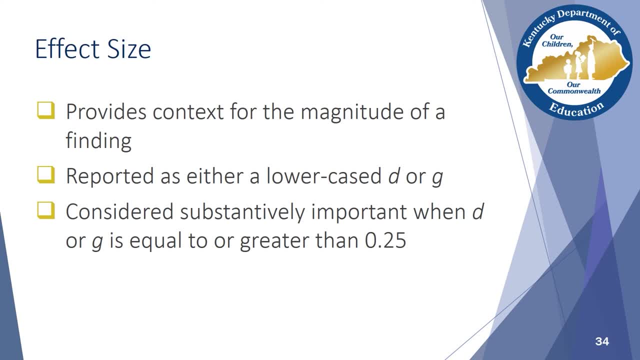 There is much debate in the scholarly world related to the interpretation of effect size. While there are many arguments for or against various attempts, the Kentucky Department of Education aligns its standards with the What Works Clearinghouse, which states that an effect size is considered substantively important when it is equal to. 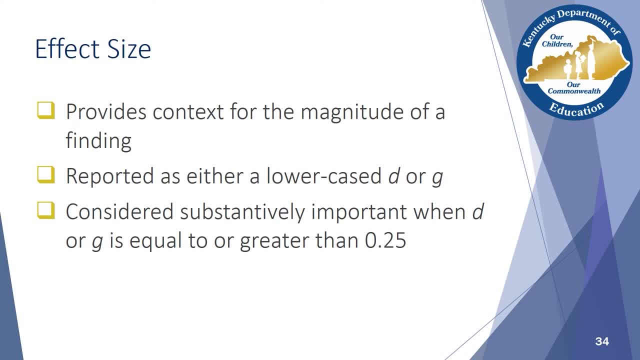 or greater than 0.25.. Effect size is an important measurement for educational decision making, but should not be the only measurement considered. It is important for education leaders to consider as much data as possible when making the decision to adopt or discontinue a practice program. 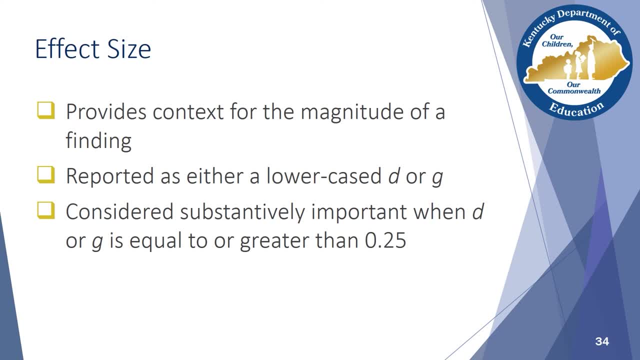 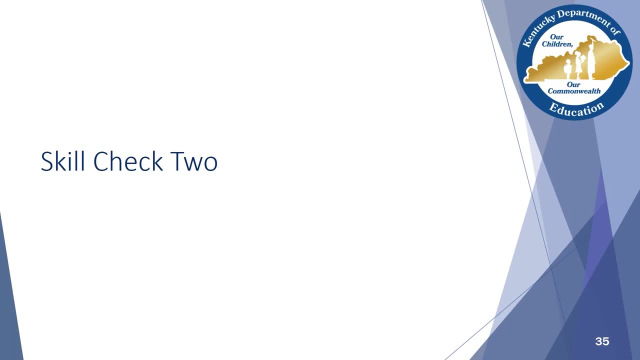 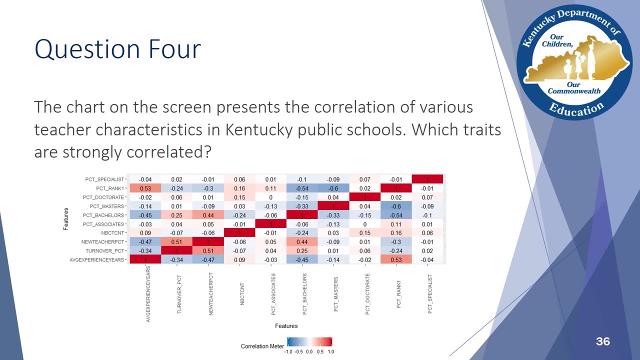 or strategy. It's time for another skill check. Just as before, the following slides will ask you to interpret the results of some statistical tests. Question 4.: The chart on the screen presents a correlation of various teacher characteristics in Kentucky public schools, Which traits are strongly correlated. Pause the webinar now. 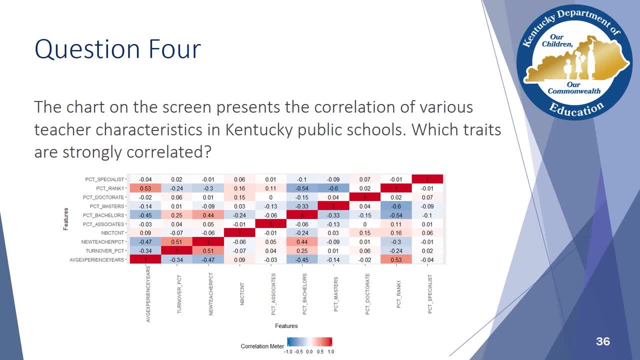 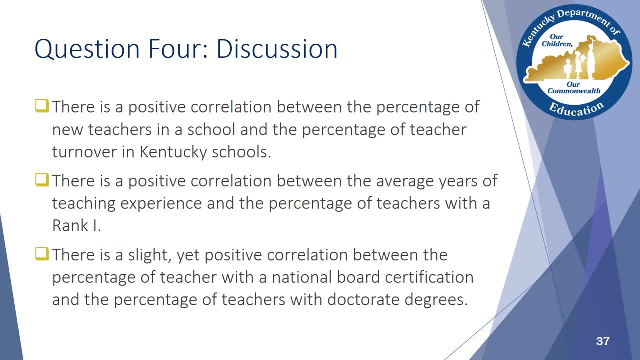 and replay when you are ready to hear the discussion. There are many different findings outlined in this chart. Let's take a look at three of them. First, we see that there is a positive correlation between the percentage of new teachers and the percentage of teacher turnover in Kentucky schools. This makes sense because if you have a 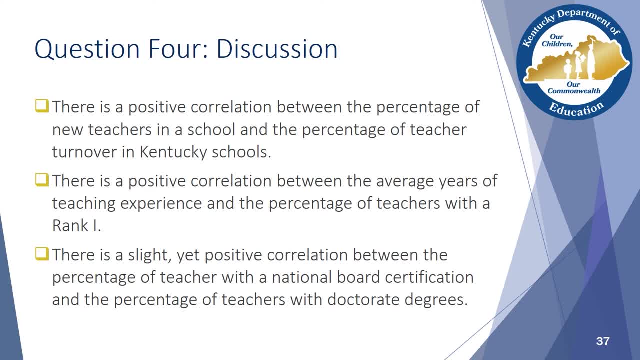 school that has a high level of teacher turnover, then they have to hire new teachers. We also see that there is a positive correlation between average years of teaching experience and the percentage of teachers in Kentucky with a rank 1.. Again, that makes sense because the longer you teach, the more likely you are to earn a rank 1.. 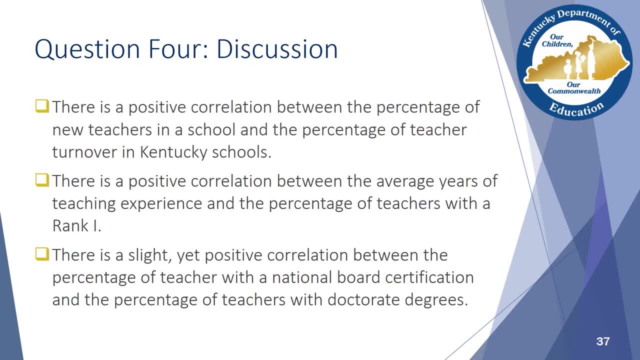 While the correlation is lower, there is a slight yet positive correlation between the percentage of teachers in Kentucky with national board certification and the percentage of teachers in Kentucky with a doctorate degree. This may suggest that teachers who pursue national board certification are more likely to pursue other forms of higher education. 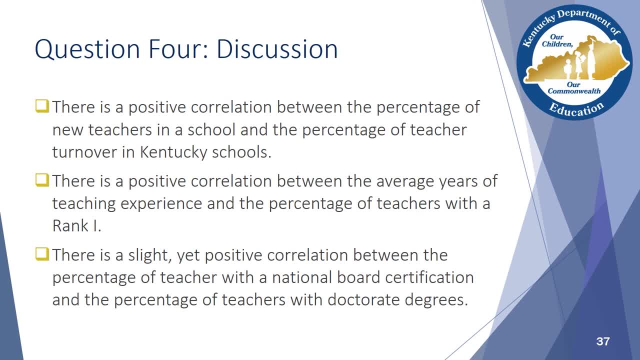 or that teachers who pursue terminal degrees are more likely to pursue other forms of professional learning. Remember, correlation does not equal causation, so we cannot say any of this for certain, but it does allow us to make some informed guesses and create a platform for our decision-making moving forward. Question 5. Below are the results: 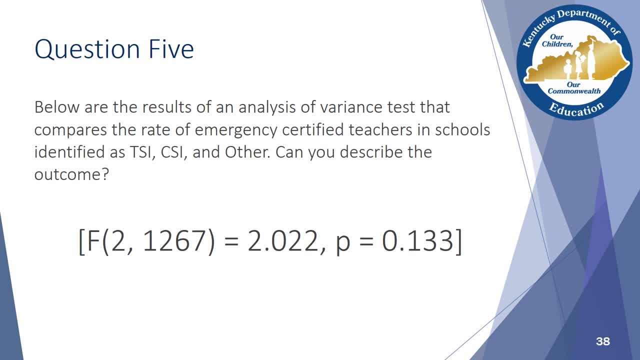 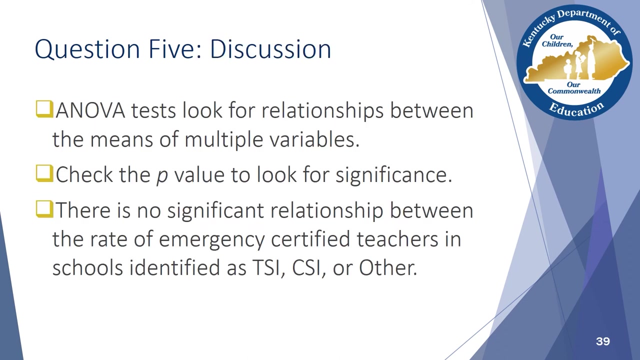 of an analysis of variance test that compares the rate of emergency certified teachers in schools identified as TSI, CSI and other. Can you describe the outcome? Pause webinar now and replay when you are ready to hear the discussion. The reporting you saw on the previous screen shows how the results of 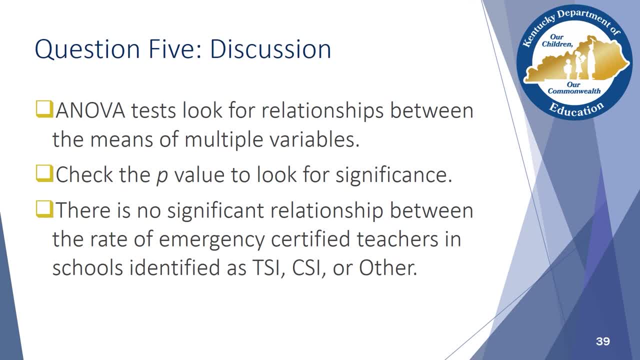 an analysis of variance tests are often reported in scholarly journals. Remember that an analysis of variance or a NOVA test looks for the relationships between the means of two or more variables. You can tell this is an ANOVA test because it is reported with a capital F If you look at the p.